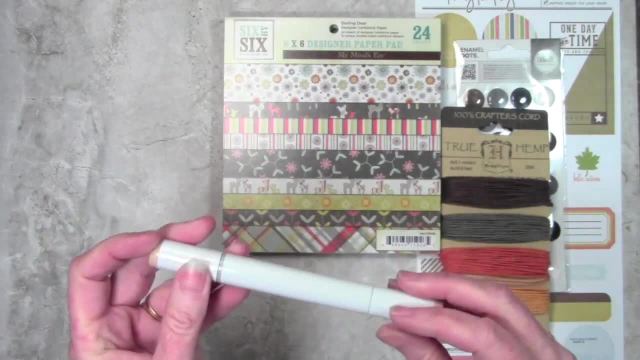 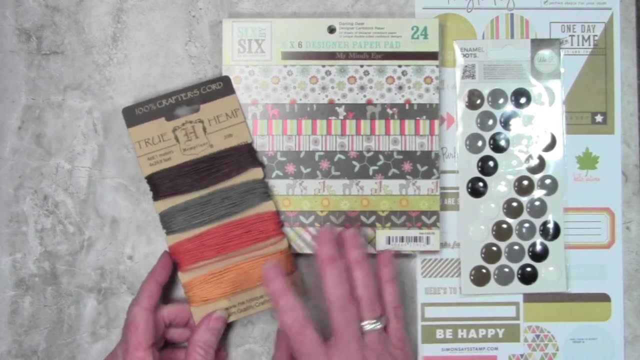 It's a really nice pale brown, And then I have this one. I also found a lot of product that's really good to complement the khaki, and those are these warm harvest tones. I think it's also fun to show you what colors you can coordinate with them, and so this is the Harvest Hemptique Cording. 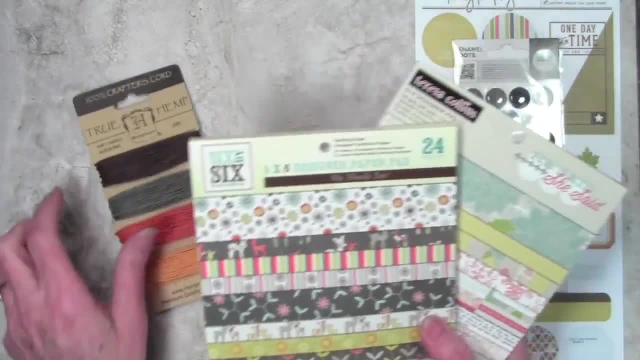 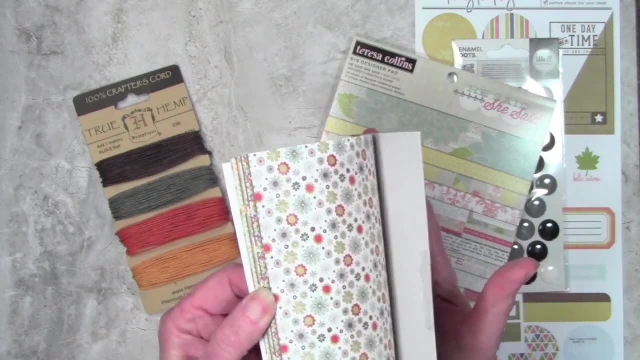 I also found a couple paper pads, and it's the 6x6 Darling Deer by Mind's Eye. It has some really nice oranges and other tones in there, especially like a little gold. I'll go ahead and flip through this. They also have a gray in here and I thought that goes really good with the khaki as well. 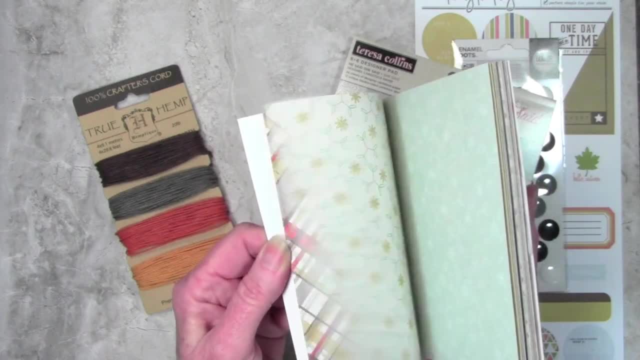 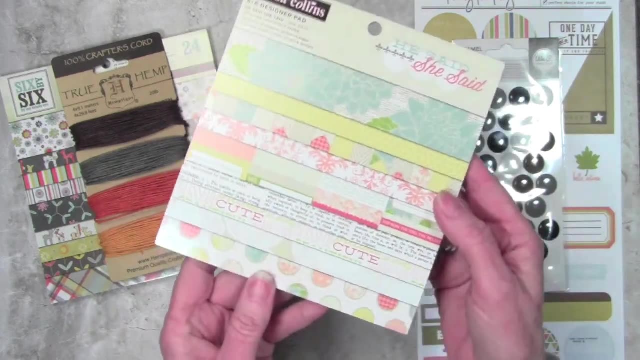 Nice, fine prints for card making And they're also double-sided front and back. The next paper pad that I found is the Teresa Collins and this is the She Said also the 6x6 pad, And these are really, really pastel colors that I thought went well with the khaki. 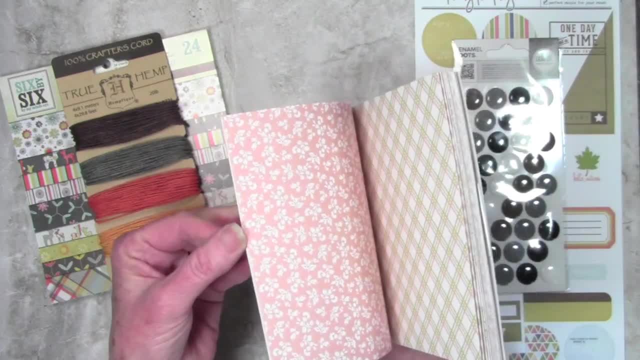 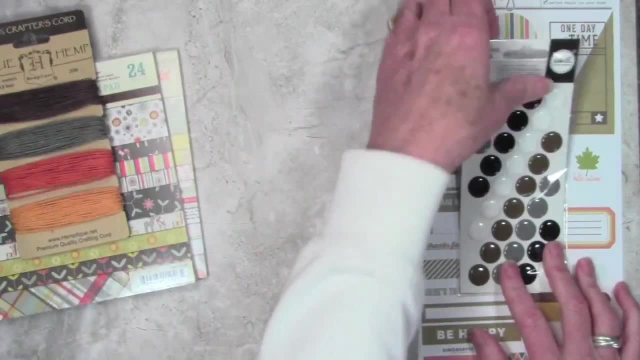 And these are also front and back, Really nice prints. Some of them are bold and some of them are really fine. So 6x6 by Teresa Collins and also my Mind's Eye, I found some really fun enamel dots. They're really large and these are. We Are Memory Keepers. 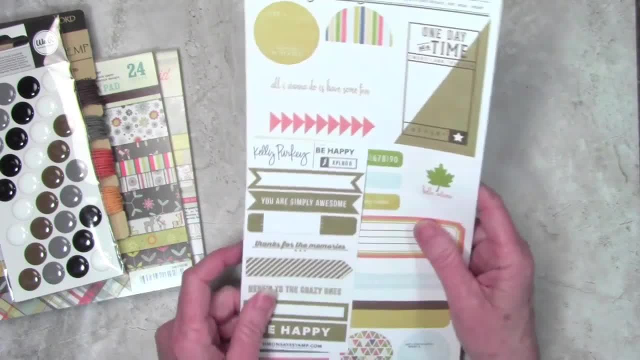 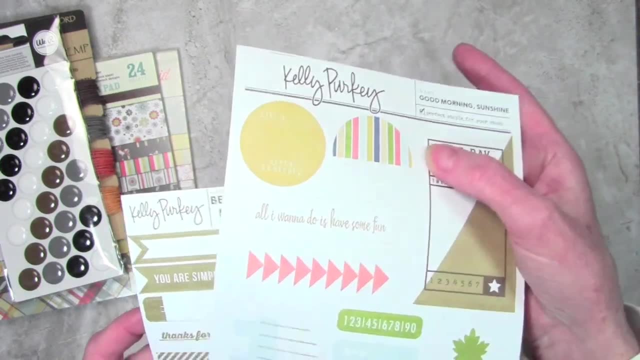 And some really neutral tones that you can mix and match with. Finally, I have some Kelly Perky stickers And the large set is a really nice guide to show you other colors that you can mix and match with your khaki color And these are really nice circles and other shapes of the stickers. 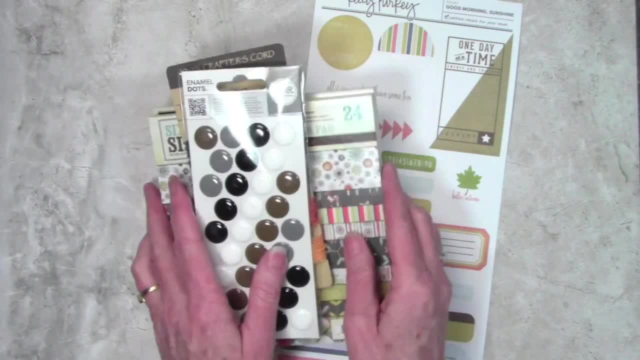 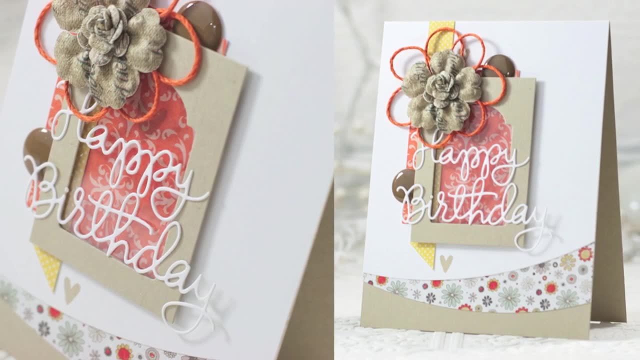 And then there's also the smaller set that is all one color and almost just a dark khaki. I did put a card together to show you how I would use the product And the color coordinates listing. I happen to really love muted colors and especially the earth tone type colors. 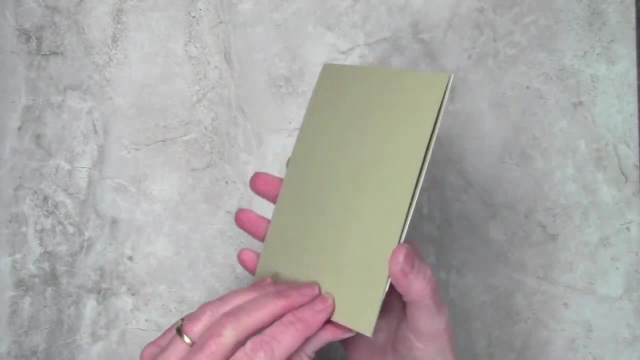 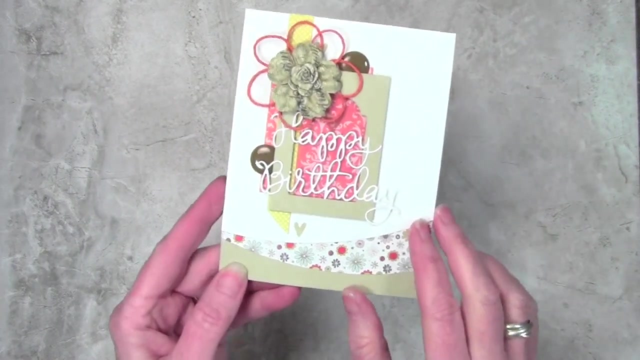 So here's my card up close. I've started with the khaki card stock and created a top folding card. Then I used the curved edge die to cut my white Neenah card stock and also a piece of the My Mind's Eye printed paper. 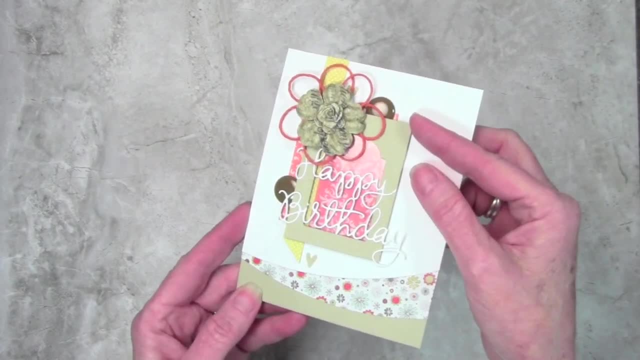 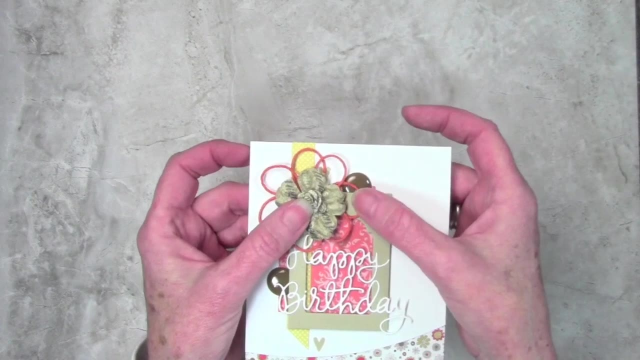 I created a little frame using one of the Simon Says Stamp dies and put some acetate inside. I've added the enamel dots and happy birthday And also a flower And loop some of that twine cord around to highlight my flower. So that is my card, using the khaki color coordinate.